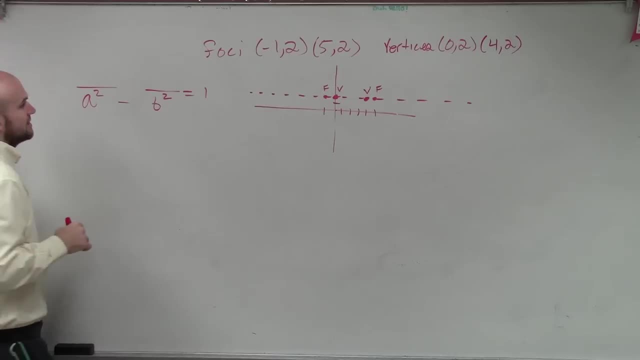 Is this at 0, 0? Sorry, No, we'll talk about that in a second. So therefore, we're going to have x minus h, squared minus y minus k. Okay, so therefore, for us to figure, okay. 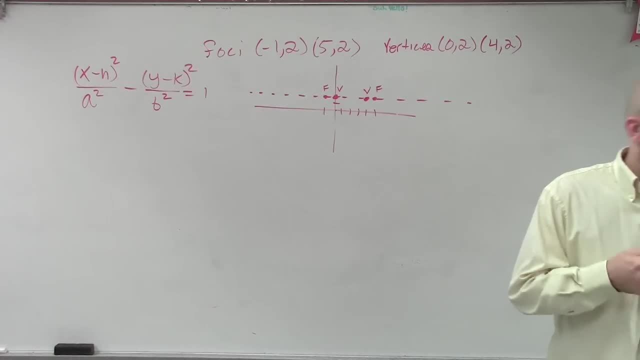 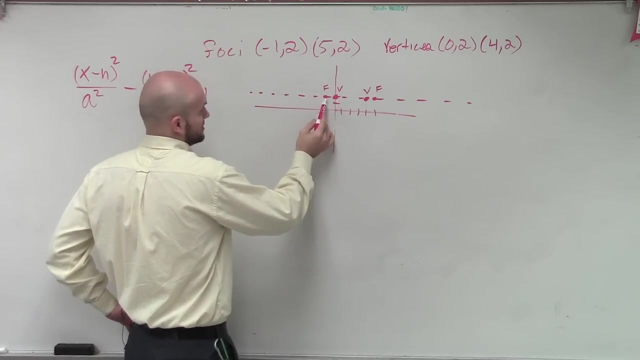 Okay, Okay, Okay, Okay, to figure out this equation, we need to know the center, we need to know a, we need to know b, right? So remember that the vertices are the exact distance from our center point. So I have vertices at zero or at negative one, two. 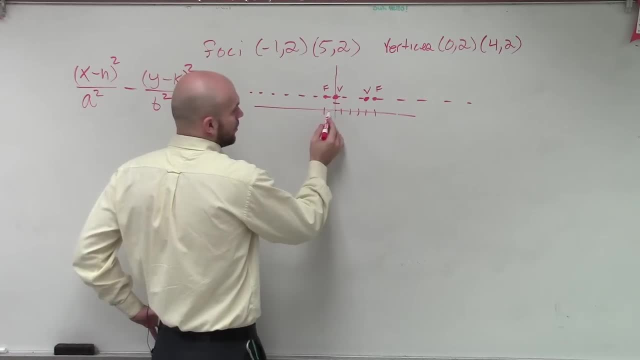 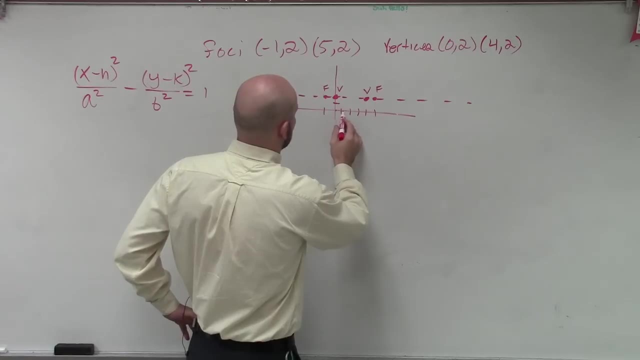 and at five count two. So how far is that distance? One, two, three, four, five, six, seven. Yeah, one, two, three, four, five. OK, One, two, three, four, five, six right. 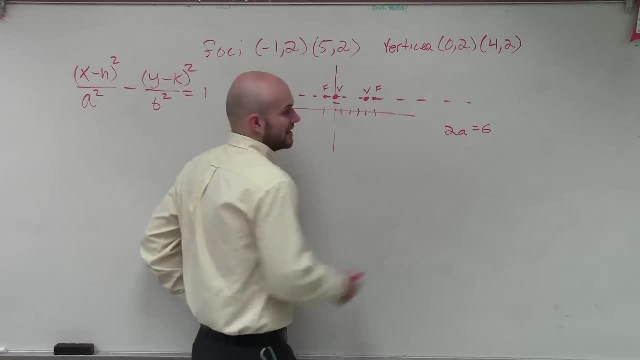 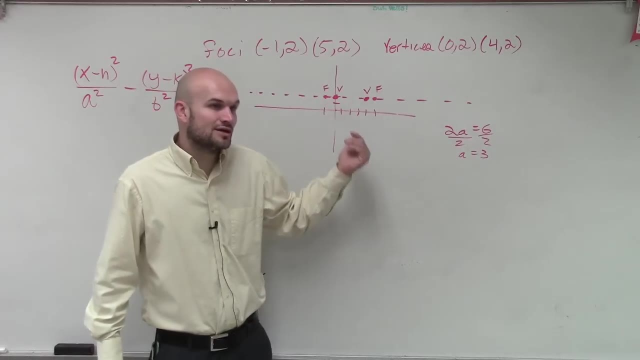 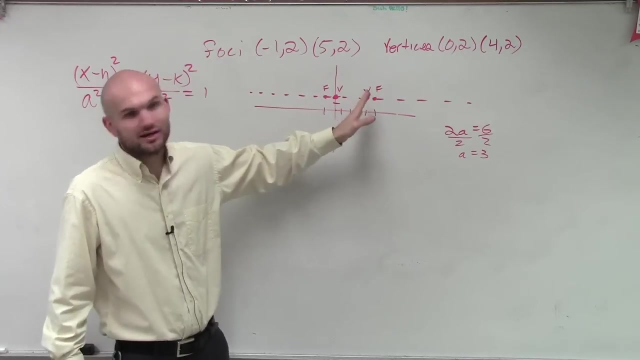 So you could say: 2a equals 6, right, So therefore my a equals 3.. That means the distance from my center to my vertices is going to be 3. 3. So therefore, if I just travel back three, 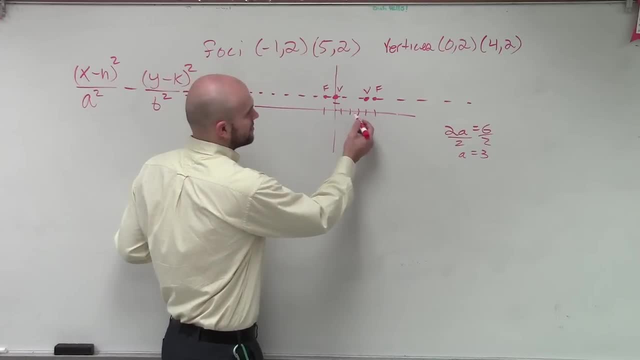 I can figure out where my center is going to be, which is 2.. 2. Where's my two vertices, One, two. oh, I was doing four, 5 minus 3.. Where are you? I was doing my foci. 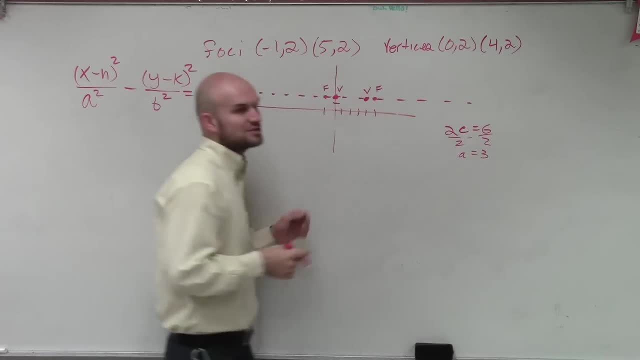 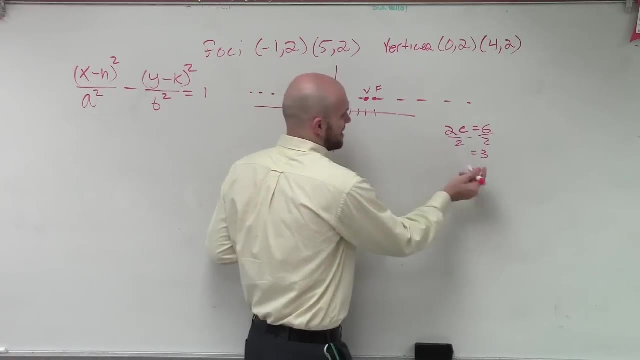 Oh, good view. That's because I was doing 2c. The distance between your two foci was 2c, which is c equals 3.. My apologies If I do a, the distance between my two vertices, which is 0, 2, and 4, 0?. 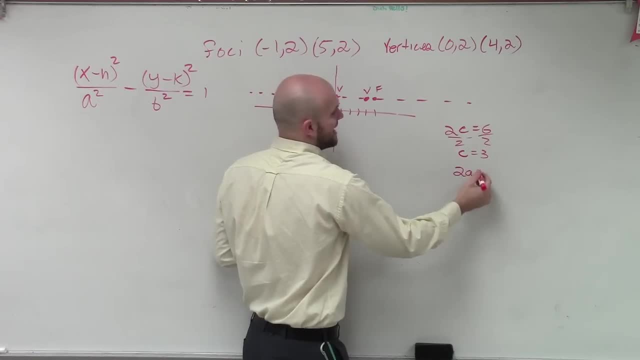 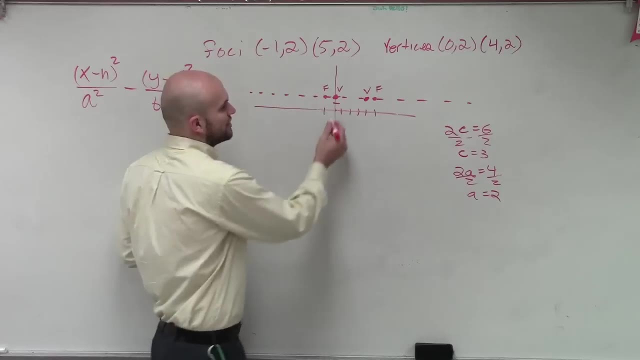 4. Was 4.. Thank you. So you could say: 2a is equal to 4, divide by 2, a equals 2.. Now again, let's go in two units from our a or from our vertices. 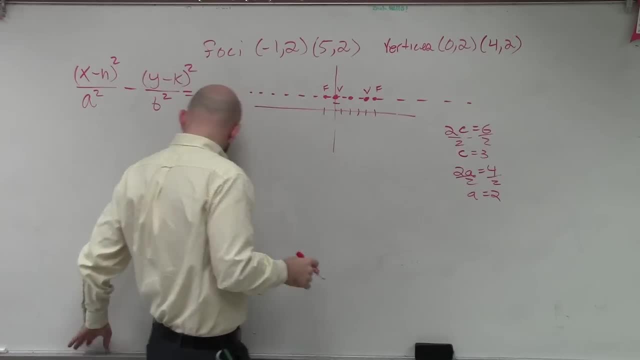 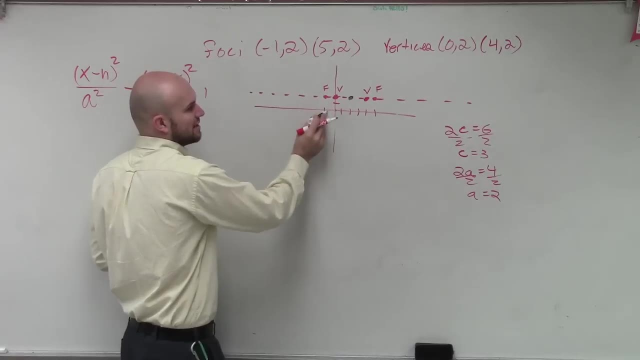 1, 2.. Let's make this a different time. 2 comma 2 is the center, And now let's go three units from your foci: 1, 2, 3.. Oh, look it, My center is going to be at 2 comma 1.. 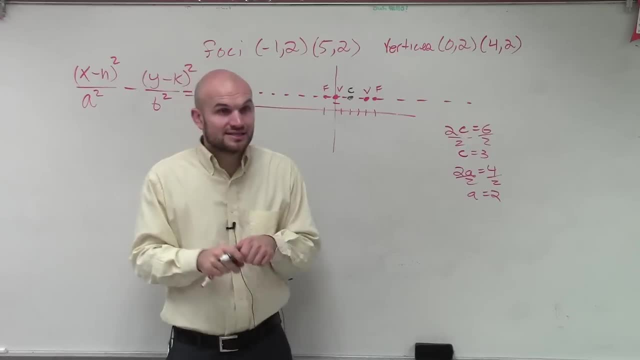 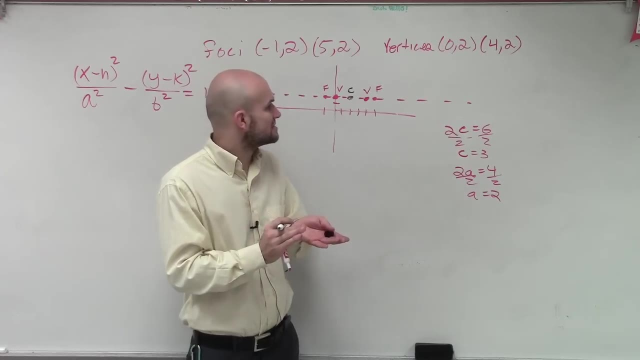 Yes, How did you find the center? Remember, the center is exactly in between your two vertices And your foci. Right It's 2 comma 2.. Yes, 2 comma 2.. Right, It's right in the middle between the two vertices. 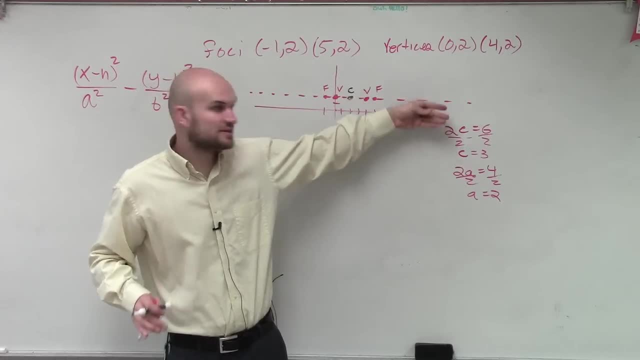 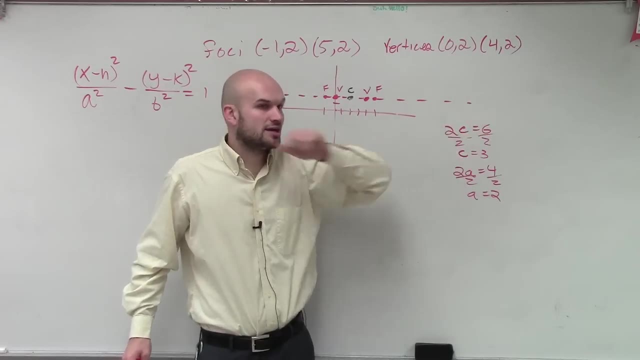 and the two foci Right. So what I did is I pretty much just found the distance between my two focis and divided it by 2.. I found the distance between my two vertices and then divided it by 2.. OK, Because it's right in the middle. 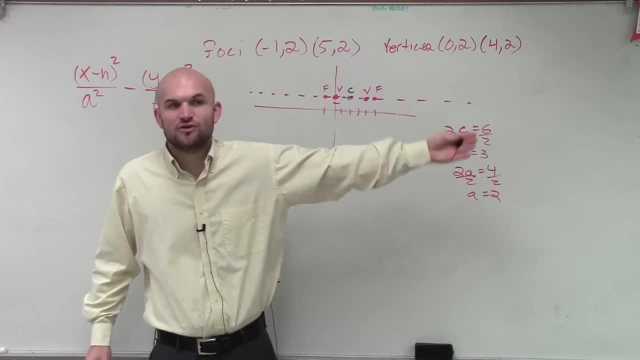 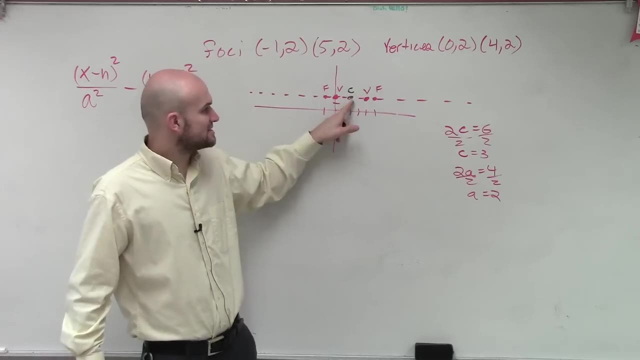 The center's right in the middle. It's equal distance to both vertices and both foci. So you just need to find that That middle, which is c, is the distance from the center to the foci. c is this distance from the center to the foci. 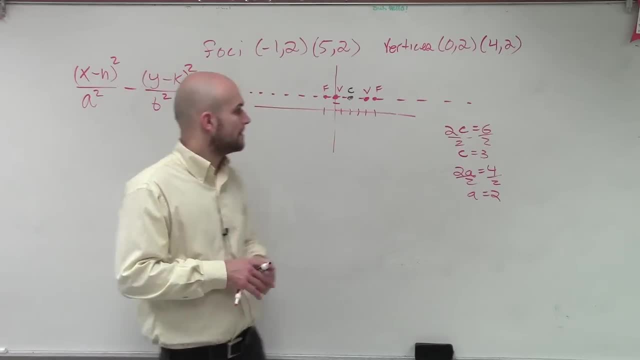 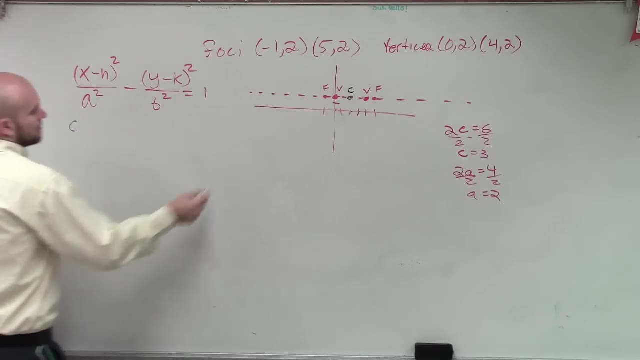 a is the distance from your center to your vertices. So now we know our center. Center is 2 comma 2, right, Very, very good. Now let's go and take a look at. so we know the center's 2 comma 2.. 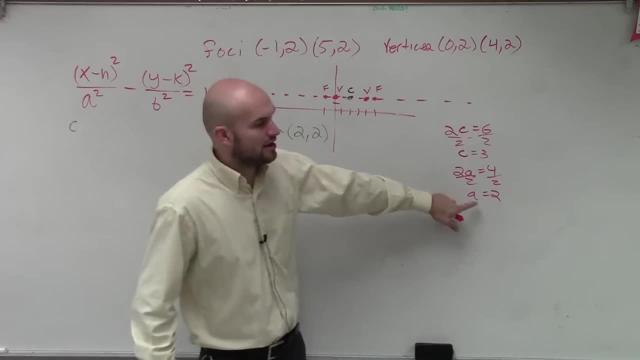 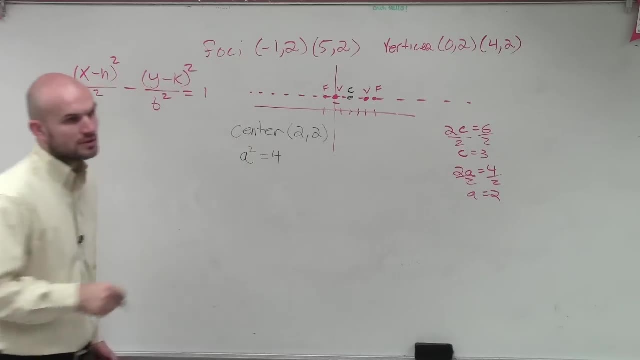 The next thing is we need to figure out what our a is. Well, we talked about a or- sorry, a squared. We know a is 2.. So, therefore, a squared is going to equal 4.. Now do we know what b squared is? 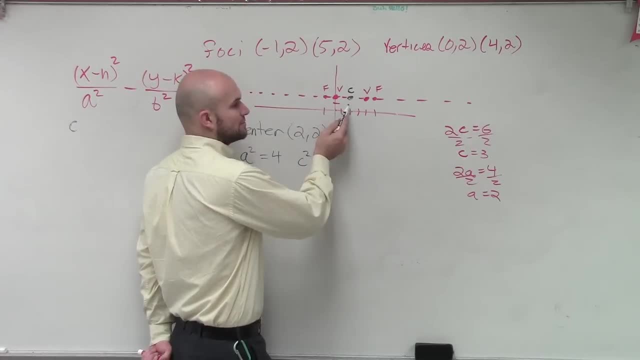 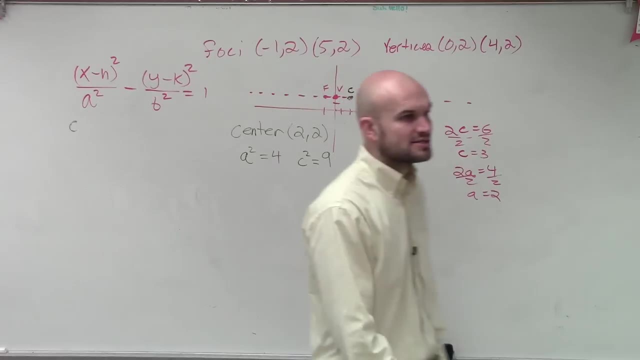 No, But do we know what c squared is? c squared is now going to be the distance, remember here. So c is 3. So c squared equals 9.. Now why is it so important for us to be able to figure out what c? 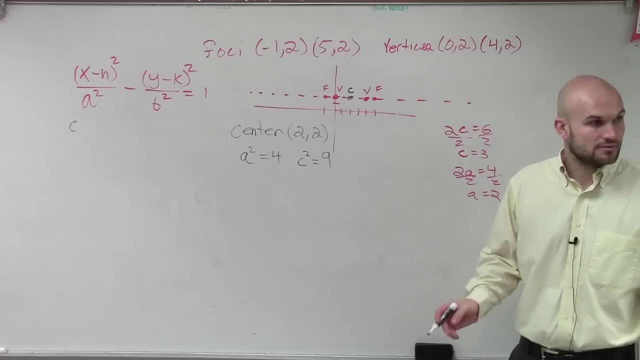 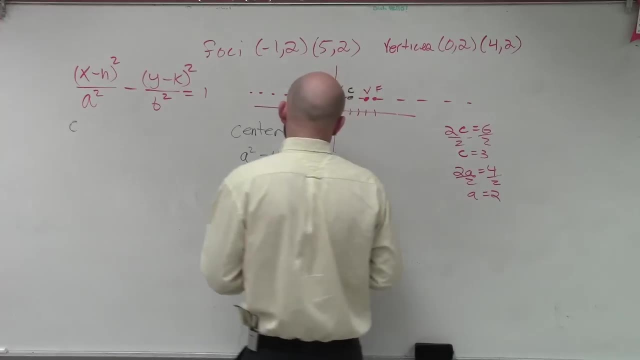 and a are, because now we can figure out what b is right. b is bigger than a, though, when you figure it out, OK, So let's go and take a look at it. So remember, in this one we're going. 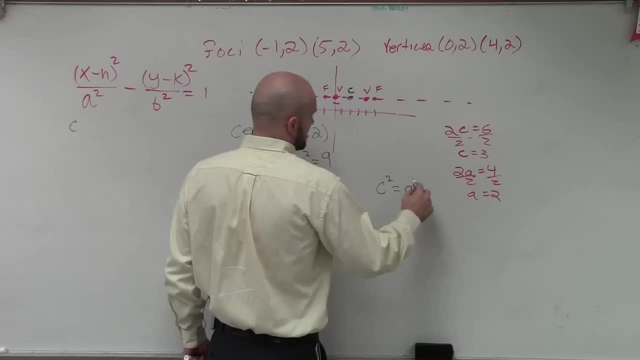 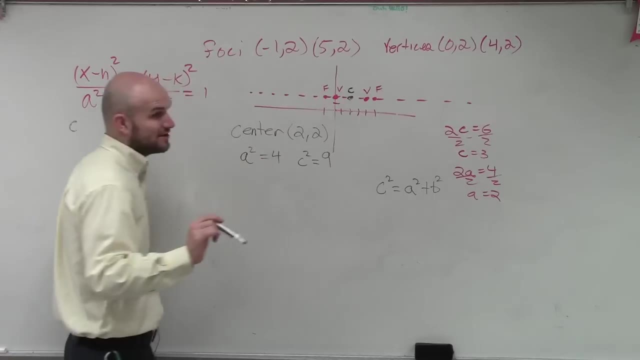 to have c squared equals a squared plus b squared, right, But remember now it's a little bit different than what we were dealing with in the last one. Your b is going to represent different values because, remember now we have this inverted right. 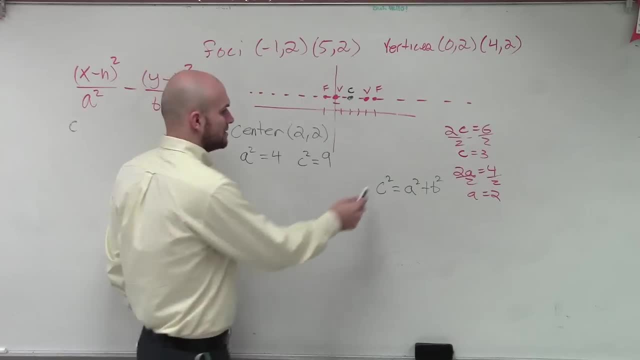 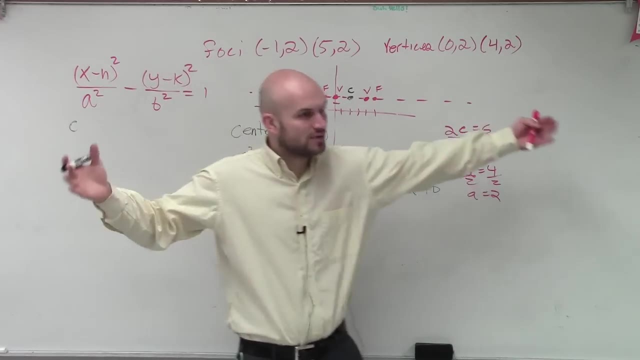 E squared, It's not opening like an ellipse Now, it's inverted, going back the other way. So therefore, remember, look at a is smaller. Remember, on an ellipse, a was your larger right Because a was outside your foci.